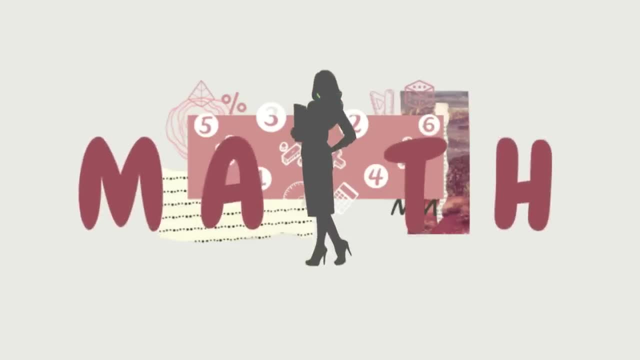 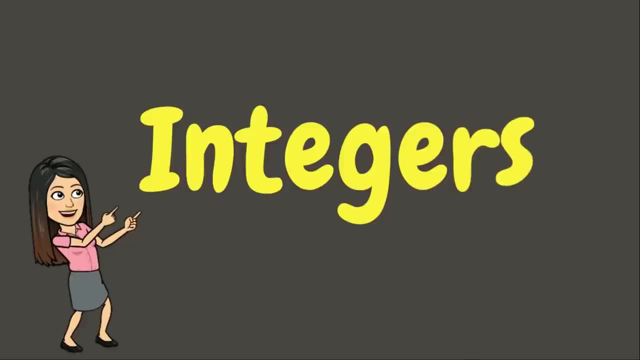 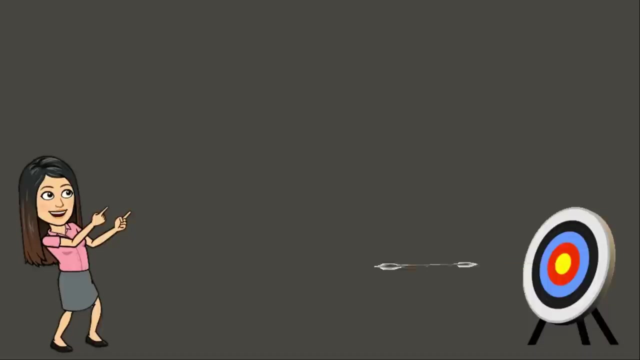 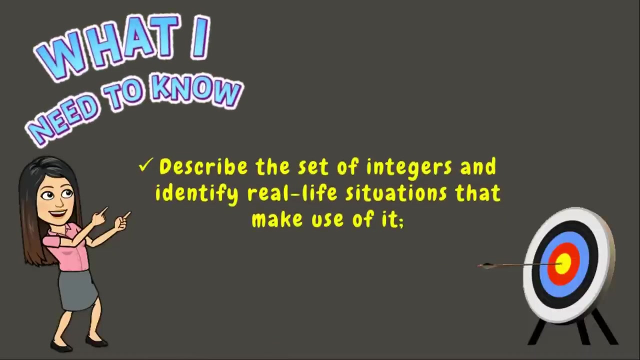 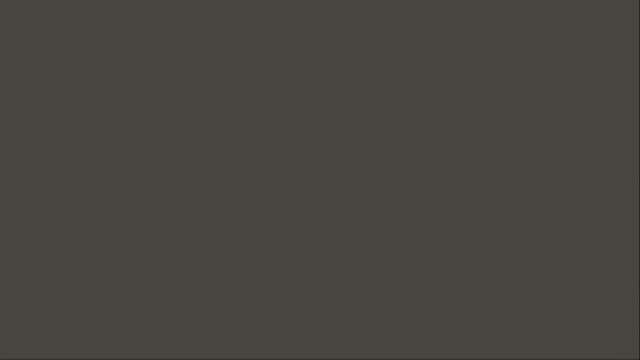 Good day students. welcome back to my classroom For today's lesson. you will learn how to describe the set of integers and identify real-life situations to make use of it and compare integers. Let us begin. Integers are whole numbers which consist of zero positive and negative numbers. Let's. 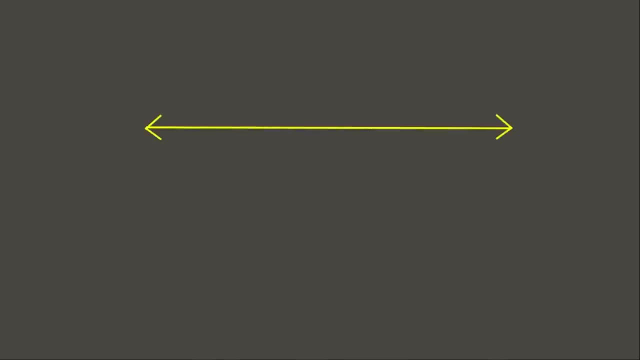 take a look at this number line. This number line is divided into right and left part by the number zero. If you are coming up with a word or an example, take a look at the above. The numbers on the right side of zero are the positive integers. These positive invoice 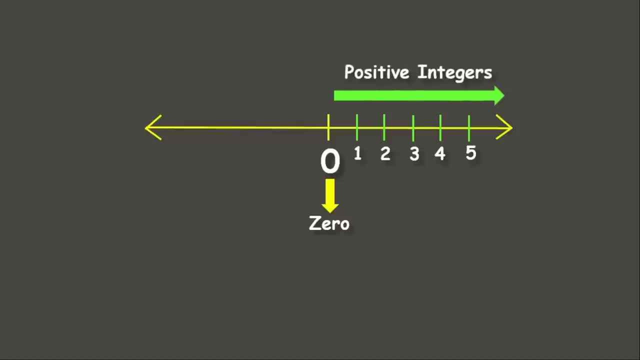 are not negative integers. They are positive integers. These positive integers can be written with or without positive sign, while the numbers to the left of zero are the negative integers, which must be written with the negative sign. Remember that integers are whole numbers. 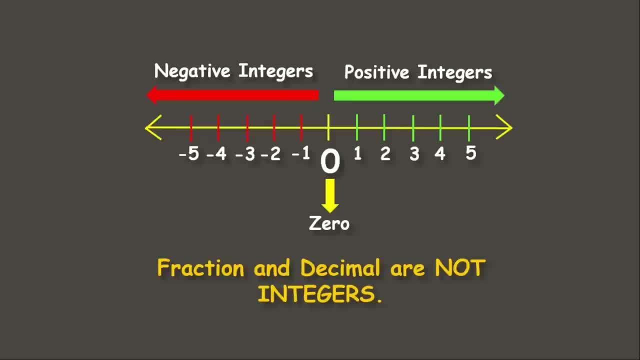 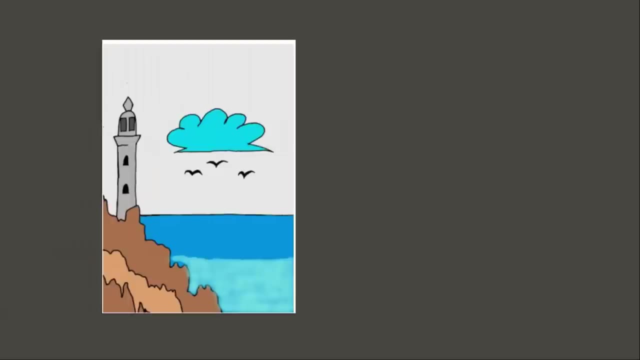 Fractions and decimals are not considered as integers. Some real-world situations can be modeled by integers. Let's take a look at this example. The sea level represents zero, While below the sea level represents negative numbers And above sea level represents by the positive numbers. 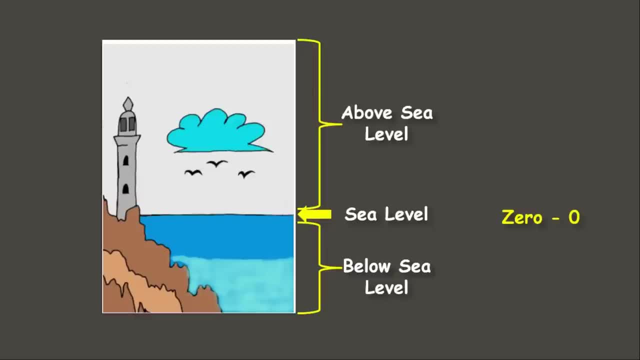 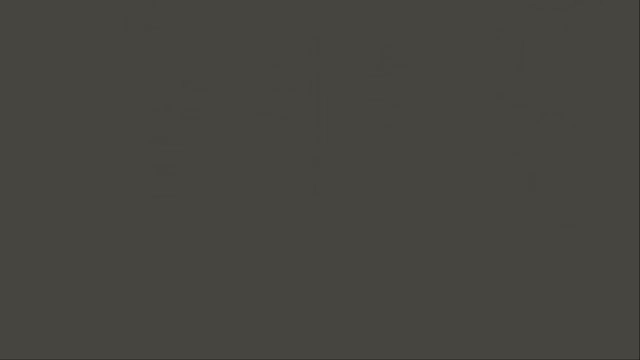 If we say 40 feet above sea level, that means it is equivalent to positive 40 feet, While if we say 40 feet below sea level, it means it is equivalent to negative 40.. Now let's try another situational phrases. 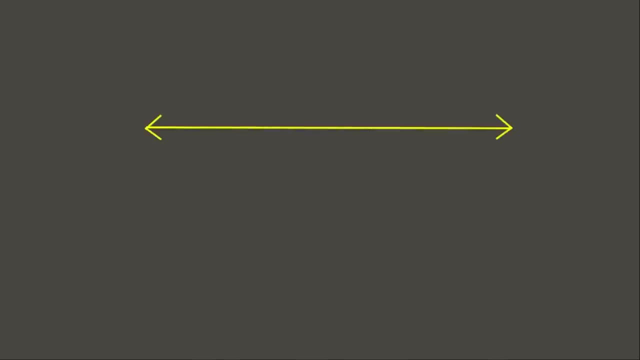 take a look at this number line. This number line is divided into right and left part by the number zero. The numbers on the right side of zero are the positive integers. These positive integers can be written with or without the positive sign, while the numbers to the left of zero 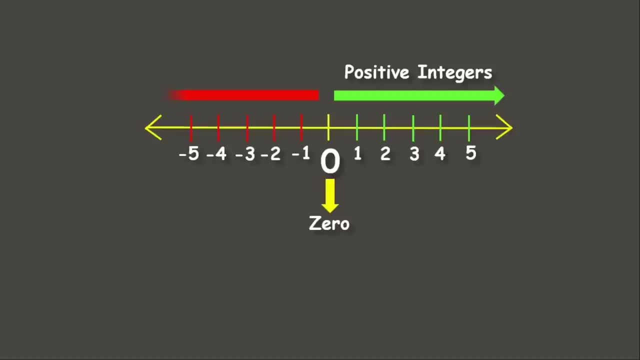 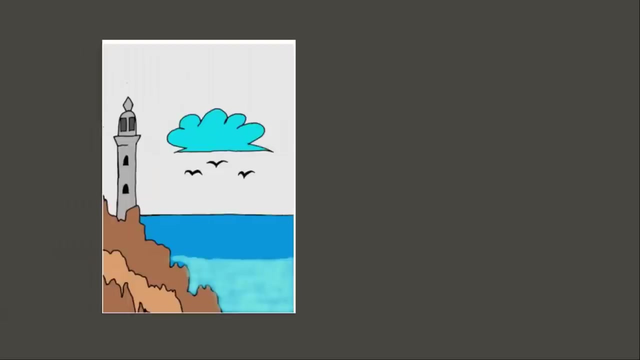 are the negative integers which must be written with the negative sign. Remember that integers are whole numbers. Fractions and decimals are not considered as integers. Some real-world situations can be modeled by integers. Let's take a look at this example. The sea level represents zero. 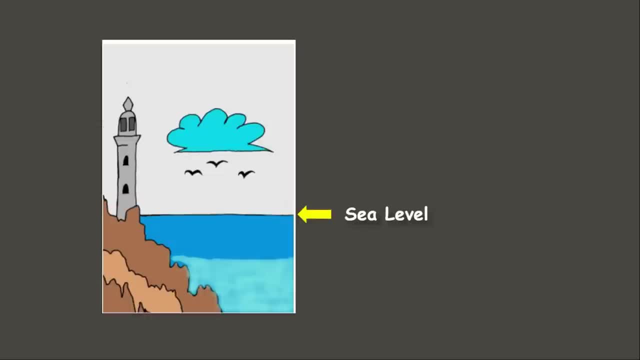 While below the sea level represents negative numbers And above sea level represents by the positive numbers. If we say 40 feet above sea level, that means it is equivalent to positive 40 feet, While if we say 40 feet below sea level, 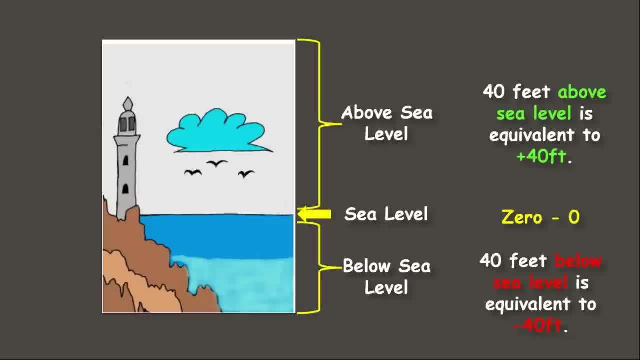 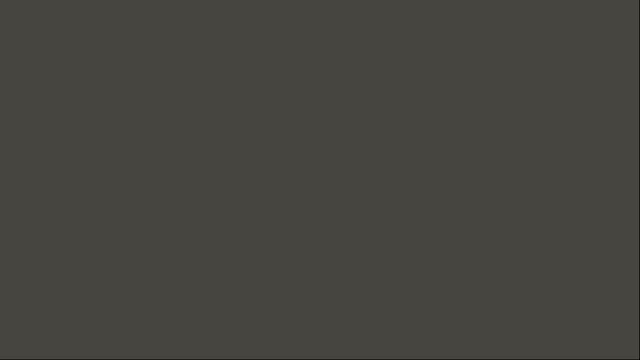 it means it is equivalent to negative 40.. Now let's try another situational phrases which can also be represented by integers. We have here 15 feet above the ground. Our clue word here is the word above, which represents positive number. 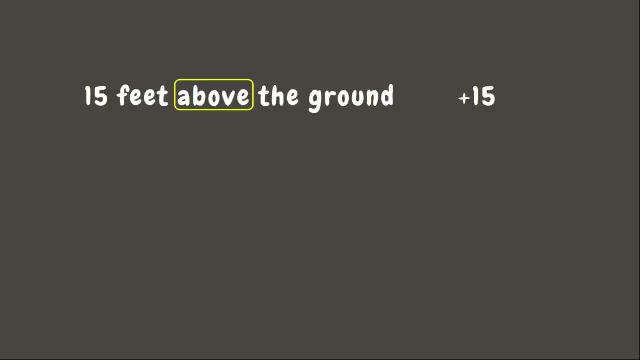 This means that it can be represented by positive 15.. Another one: We have 10 floors up. Our key word here is the word up. It means that it is positive 10.. Next one: We have 5 steps backwards. 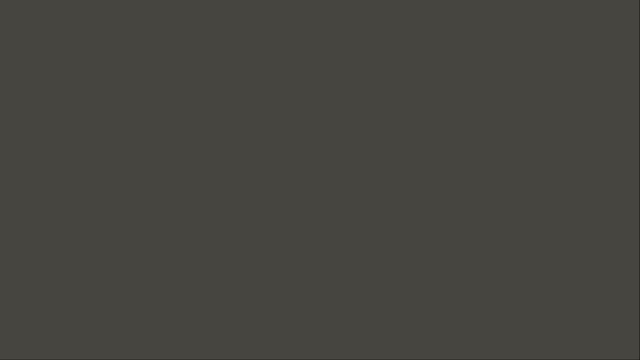 which can also be represented by integers. We have here 15 feet above the ground. Our clue word here is the word above, which represents positive number. This means that it can be represented by positive 15.. Another one: We have 10 floors up. 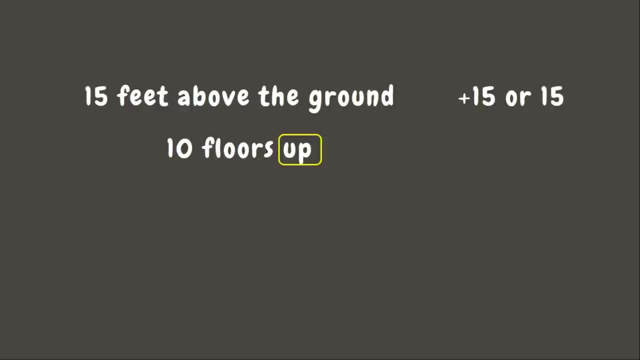 Our key word here is the word up. It means that it is positive 10.. Next one: We have 5 steps backward. Our clue word here is the word backward. It means that we are going to move 5 steps backward, So that is negative 5.. 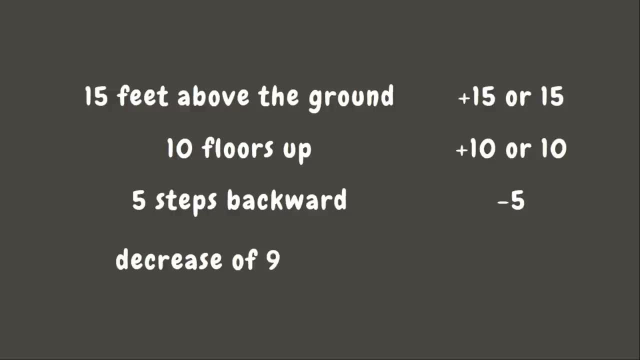 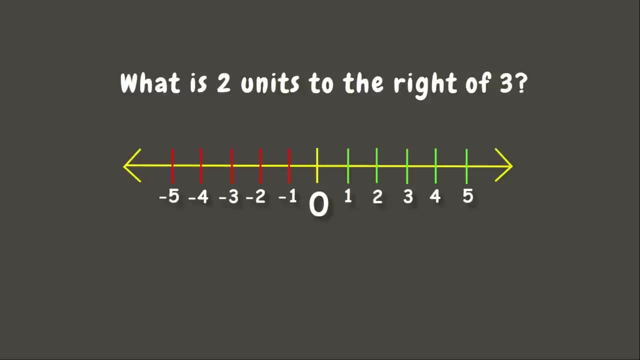 And, lastly, we have decrease of 9 points. It can be represented by negative 9.. Wonderful. Now, if we are asked this question: What is 2x? It is 2 units to the right of 3.. It means that we need to move 2 units, or 2 times, to the right of the number 3.. 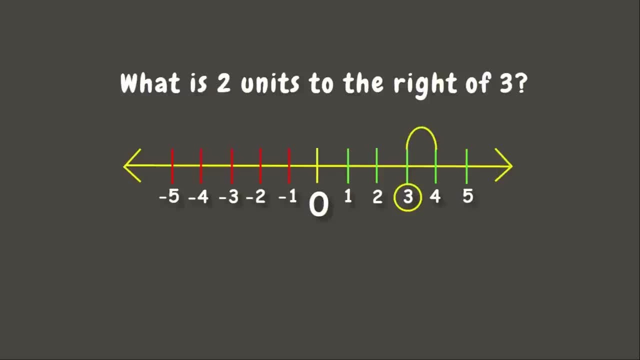 Let's try it There. It means 2 units to the right of 3 is positive 5.. This also represents addition, Where when we add 2, and 3, that gives us positive 5.. Another example: What is 5 units to the left of 0?? 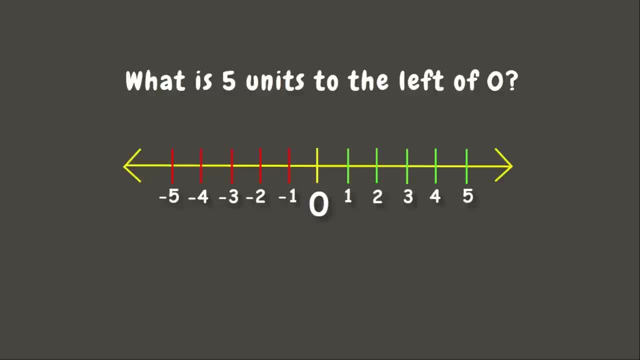 This means that we need to move 5 times to the left from 0. So let's try, Great job. So that is negative 5.. This also represents subtraction, Where 0 minus 5 is negative 5.. Now let's learn how to compare integers. 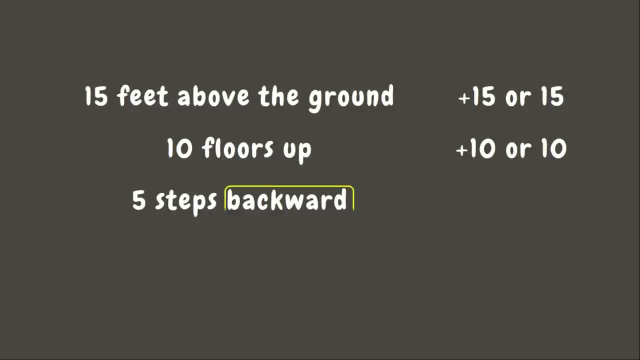 Our clue word here is the word backwards. It means that we are going to move 5 steps backwards, So that is negative 5.. And lastly, we have the crease of 9 points. It can be represented by negative 9.. 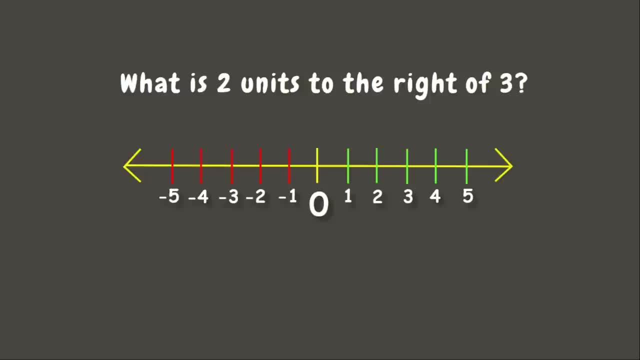 Wonderful. Now, if we are asked this question: What is negative 9?? What is 2 units to the right of 3?? It means that we need to move 2 units, or 2 times, to the right of the number 3.. 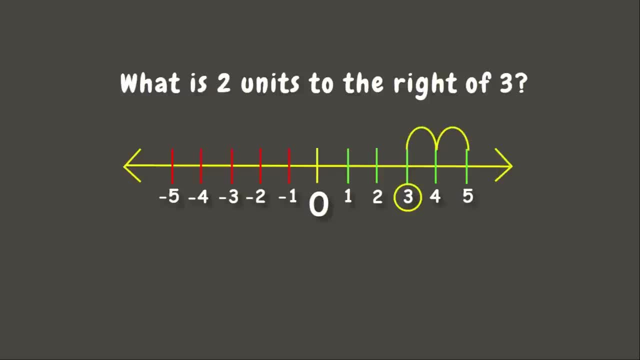 Let's try it There. It means 2 units to the right of 3 is positive 5.. This also represents addition, Where when we add 2, and 3, that gives us positive 5.. Another example: What is 5 units to the left of 0?? 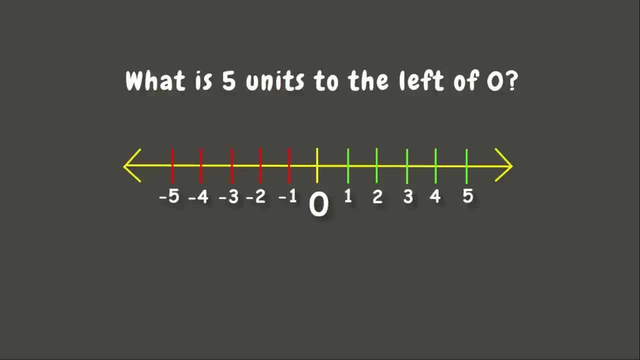 This means that we need to move 5 times to the left from 0. So let's try, Great job. So that is negative 5.. This also represents subtraction, Where 0 minus 5 is negative 5.. Now let's learn how to compare integers. 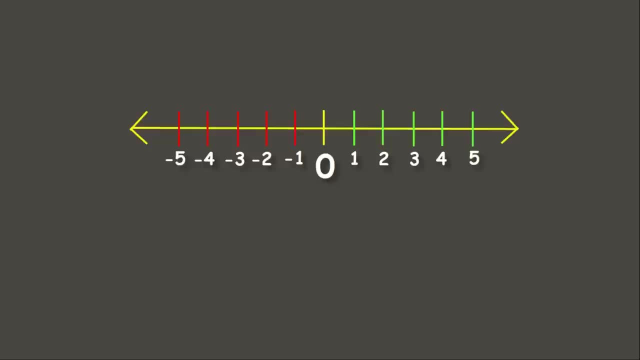 In comparing integers, we need to understand that the numbers to the right of 0 gets bigger and bigger, While the numbers to the left of 0 get smaller and smaller. Therefore, 0 is greater than negative numbers, but less than positive numbers. 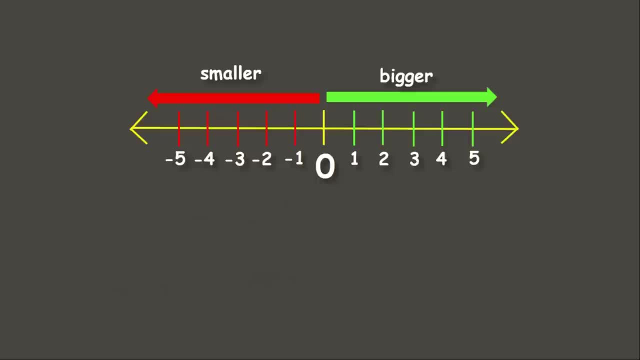 Let's try an example. Let's compare 0 and negative 5.. Since negative 5 is a negative integer and it can be found to the left of 0, this means that 0 is greater than negative 5.. Let's have another example. 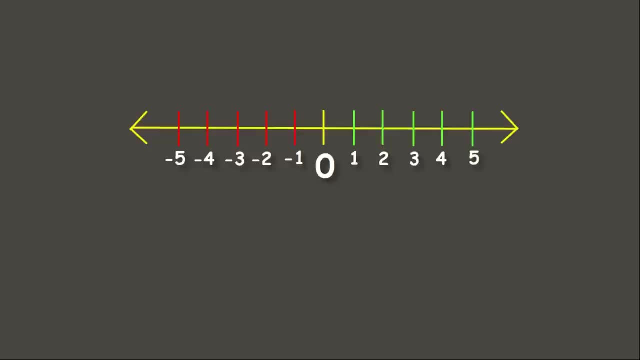 In comparing integers, we need to understand that the numbers to the right of 0 gets bigger and bigger, While the numbers to the left of 0 get smaller and smaller. Therefore, 0 is greater than negative numbers, but less than positive numbers. 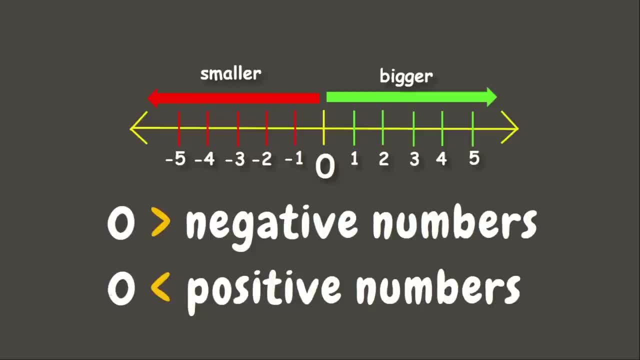 Let's try an example. Let's compare 0 and negative 5.. Since negative 5 is a negative integer and it can be found to the left of 0, this means that 0 is greater than negative 5.. Let's have another example. 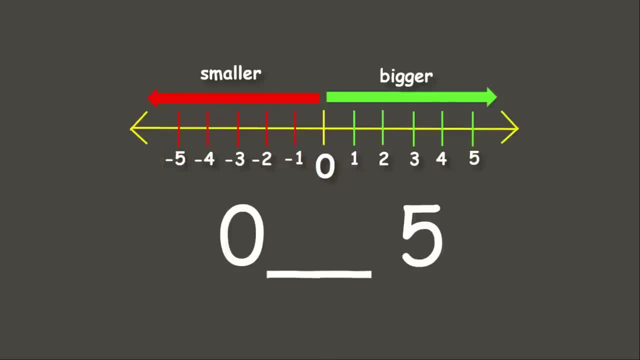 Let's compare 0 and positive 5.. Since 5 here is positive and it can be found to the right of 0,, this means that 0 is less than positive 5. Awesome. We also need to understand that all positive numbers. 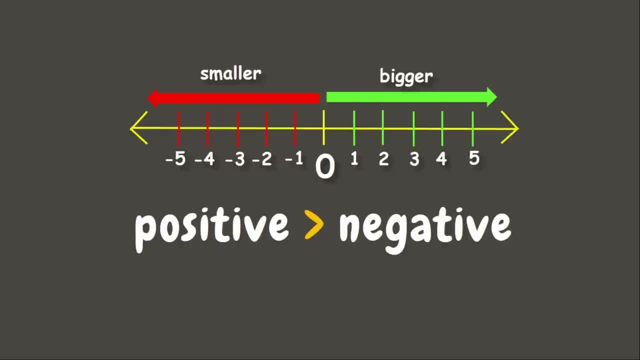 are greater than negative numbers. It means that negative numbers are less than positive numbers. Let's have an example. Let's compare positive 3 and negative 5.. When we take a look at here, it seems that negative 5 is greater than positive 3.. 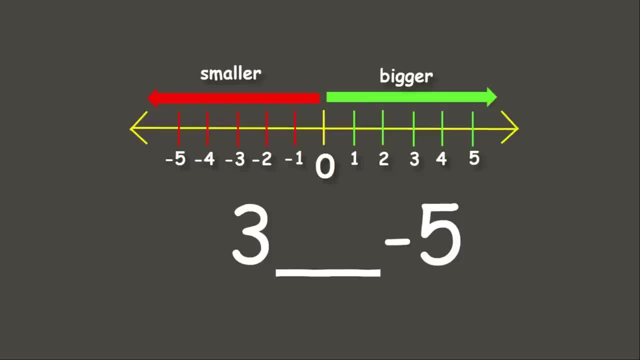 But since all positive numbers are greater than negative numbers, it means that positive 3 is greater than negative 5.. Let's have another one. This time, let us compare negative 4 and positive 1.. Again, all negative numbers are less than positive numbers. 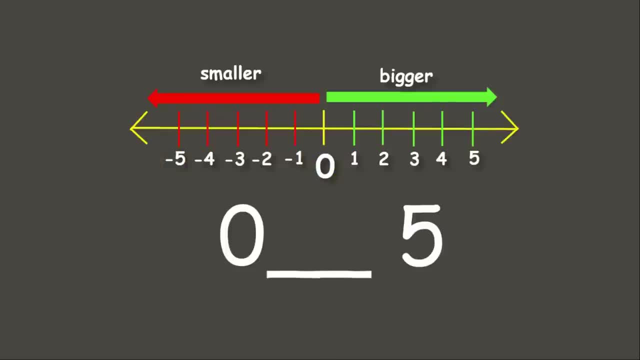 Let's compare 0 and positive 5.. Since 5 here is positive and it can be found to the right of 0,, this means that 0 is less than positive 5. Awesome. We also need to understand that all positive numbers. 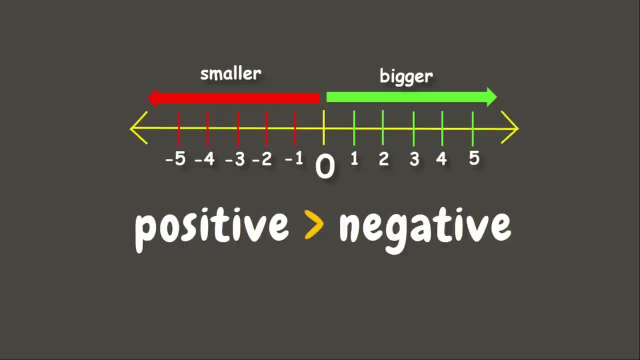 are greater than negative numbers. It means that negative numbers are less than positive numbers. Let's have an example. Let's compare positive 3 and negative 5.. When we take a look at here, it seems that negative 5 is greater than positive 3.. 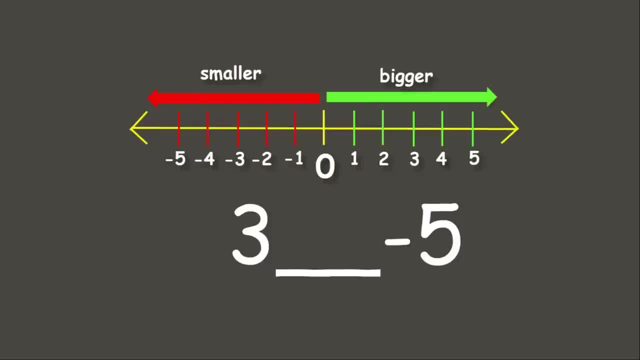 But since all positive numbers are greater than negative numbers, it means that positive 3 is greater than negative 5.. Let's have another example. This time, let us compare negative 4 and positive 1.. Again, all negative numbers are less than positive numbers. 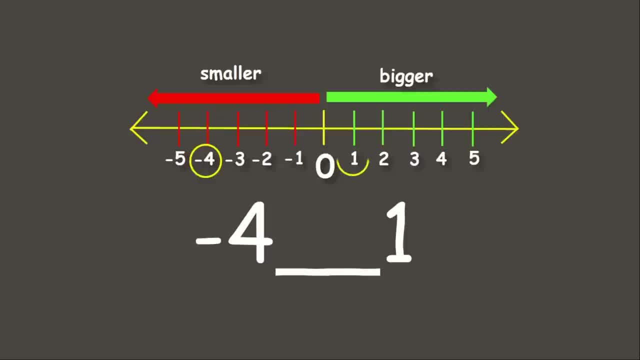 This means that negative 4 is less than positive 1.. Now let's have another example. What about we compare positive 18 and negative 25?? Since all positive numbers are greater than negative numbers, it means that positive 18 is greater than negative 25.. 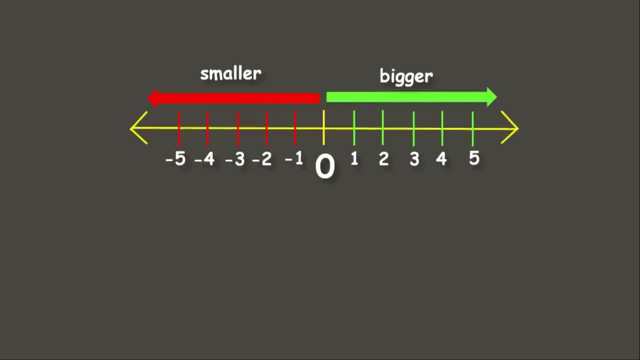 Awesome. Now let's go to another one. Now, what if we are comparing negative numbers? Since negative numbers get smaller and smaller, it means that the bigger the number, the smaller it is. Sounds confusing, right? Let's have an example. 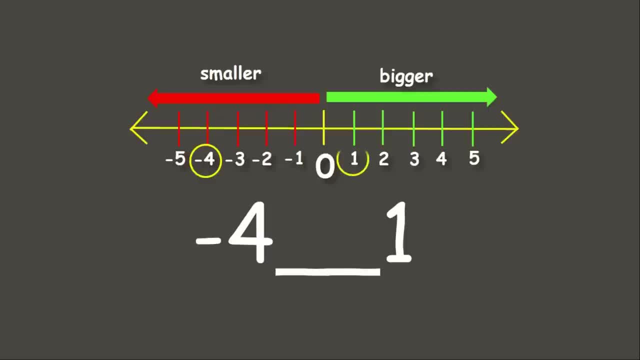 This means that negative 4 is less than positive 1.. Now let's have another one. What about we compare positive 18 and negative 25?? Since all positive numbers are greater than negative numbers, it means that positive 18 is greater than negative 25.. 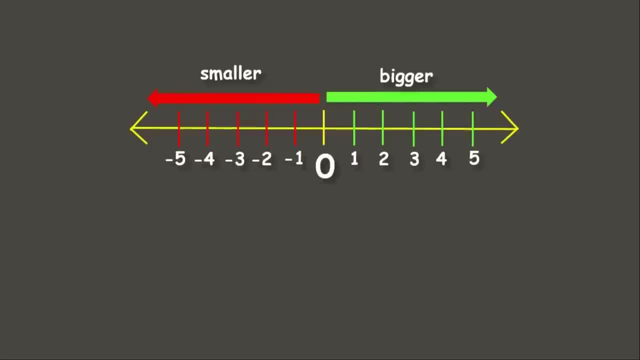 Awesome. Now let's go to another one. Now, what if we are comparing negative numbers? Since negative numbers get smaller and smaller, it means that the bigger the number, the smaller it is. Sounds confusing, right? Let's have an example. 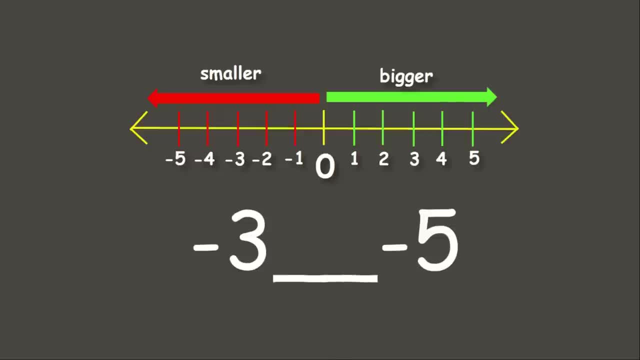 Let us compare negative 3 and negative 5.. It seems that negative 5 is greater than negative 3. But here negative 3 is closer to number 0. This means that negative 3 is greater than negative 5.. Let's have another example. 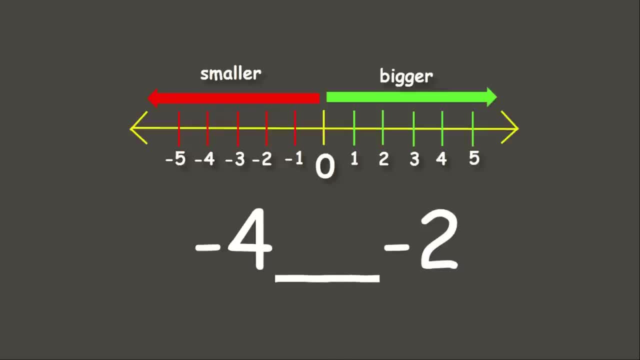 Let us compare negative 4 and negative 2.. Since negative 4 is bigger than negative 2,, it means that negative 4 is less than negative 2.. Great job, How about this one Great job. Negative 40 is less than negative 21.. 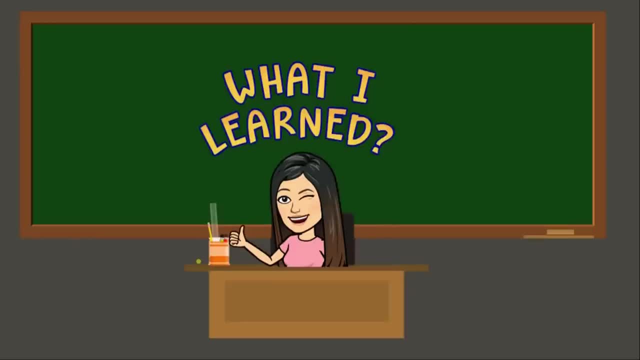 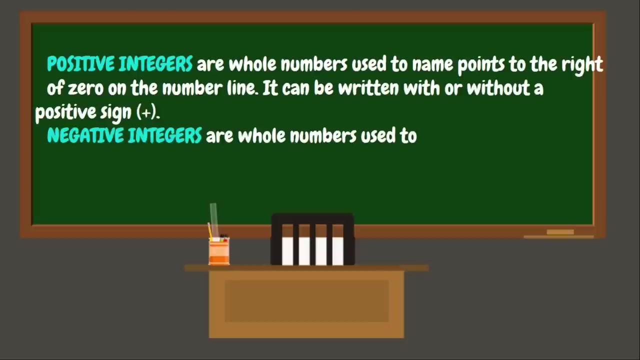 Wonderful, Great job, students. You made it. Now, here are the things that you learned today. You can find the answer in this video. In this video, we'll talk about the main problems of negative numbers. However, you won't need 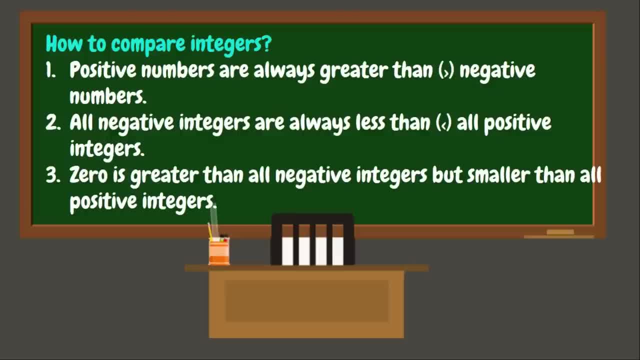 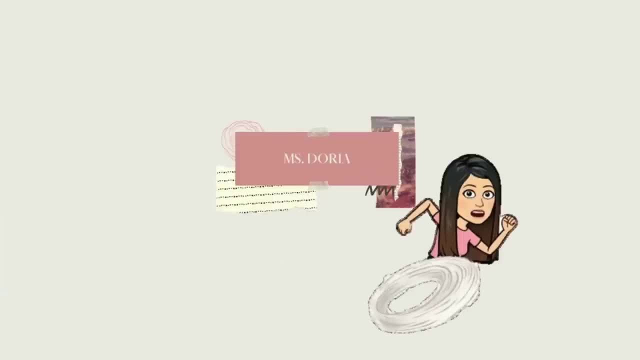 negative numbers to solve any of these problems. Instead, let's start with negative numbers first. The answer is negative 1.. Negative 2 is the most common and most common number in the class. It is the last number in this class. You have finished.